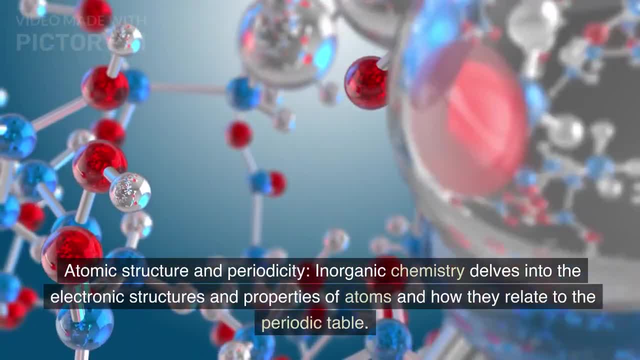 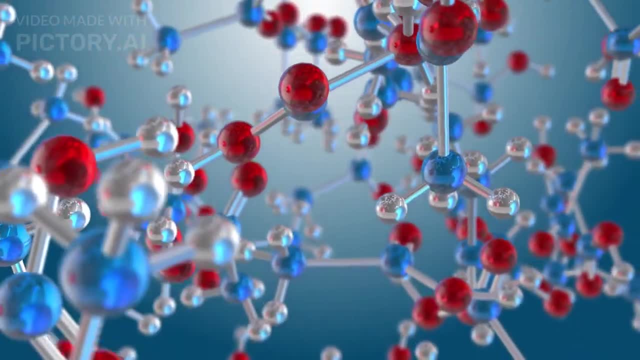 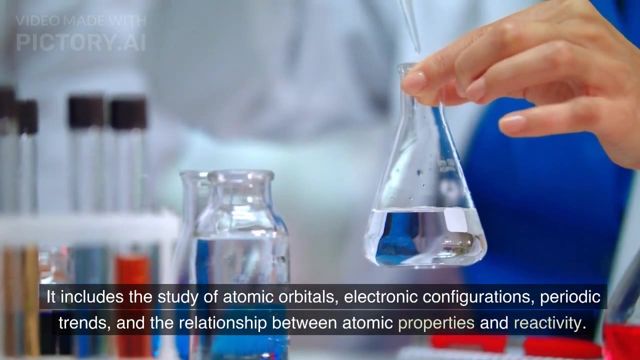 1. Atomic Structure and Periodicity. Inorganic chemistry delves into the electronic structures and properties of atoms and how they relate to the periodic table. It includes the study of atomic orbitals, electronic configurations, periodic trends and the relationship between atomic 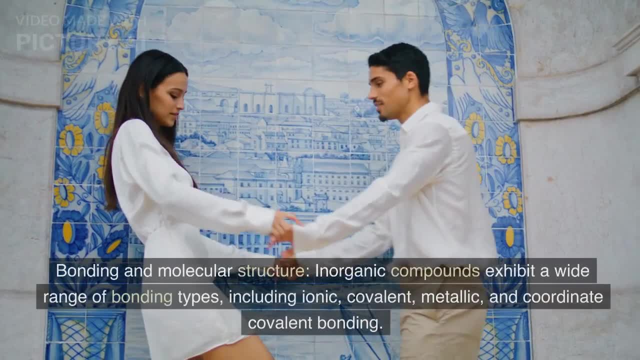 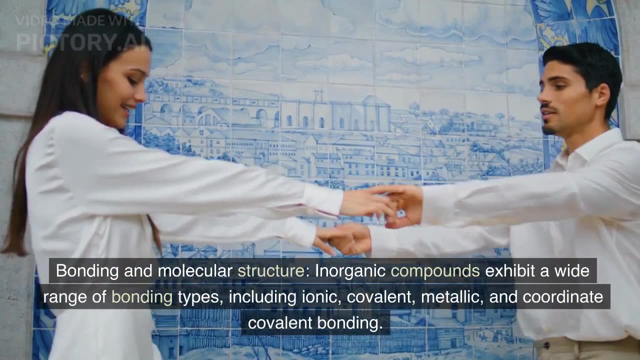 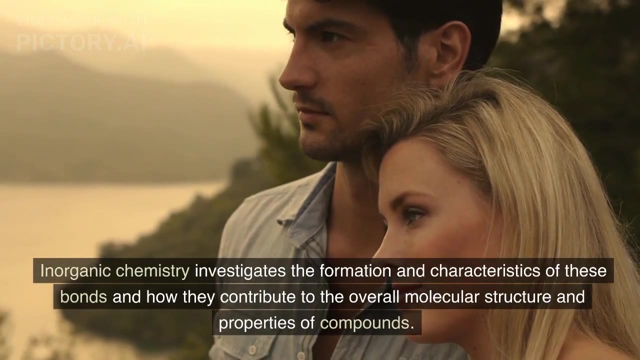 properties and reactivity. 2. Bonding and Molecular Structure. Inorganic compounds exhibit a wide range of bonding types, including ionic, covalent, metallic and coordinate-covalent bonding. Inorganic chemistry investigates the formation and characteristics of these bonds. 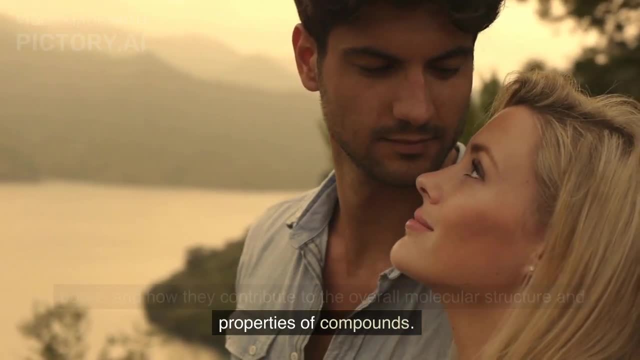 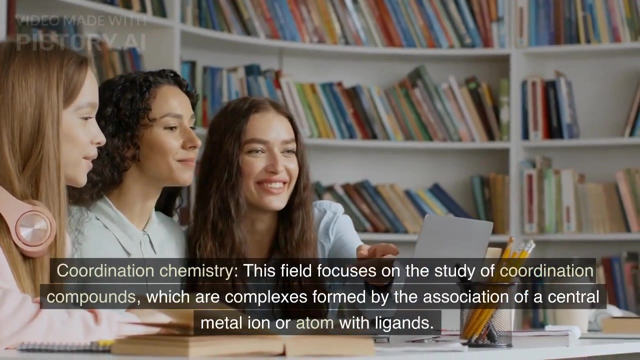 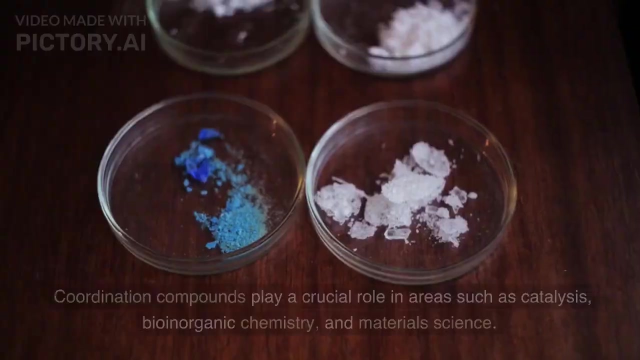 and how they contribute to the overall molecular structure and properties of compounds. 3. Coordination Chemistry: This field focuses on the study of coordination compounds, which are complexes formed by the association of a central metal ion or atom with ligands. Coordination compounds play a crucial role in areas such as catalysis. 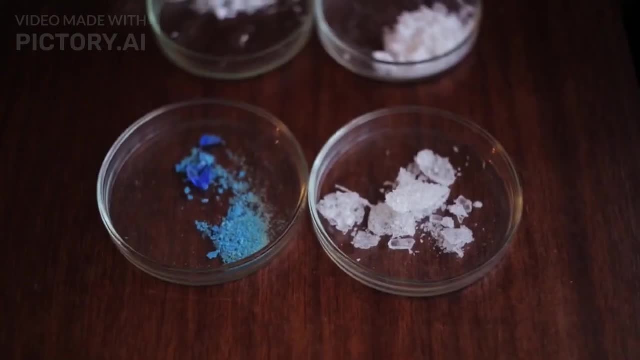 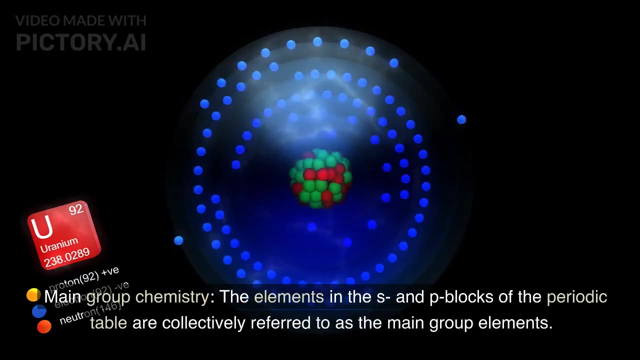 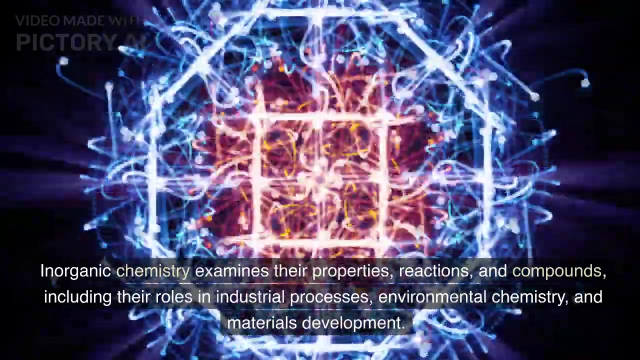 bio-inorganic chemistry and materials science. 4. Main Group Chemistry. The elements in the S&P blocks of the periodic table are collectively referred to as the main group elements. Inorganic chemistry examines their properties, reactions and compounds, including their roles. 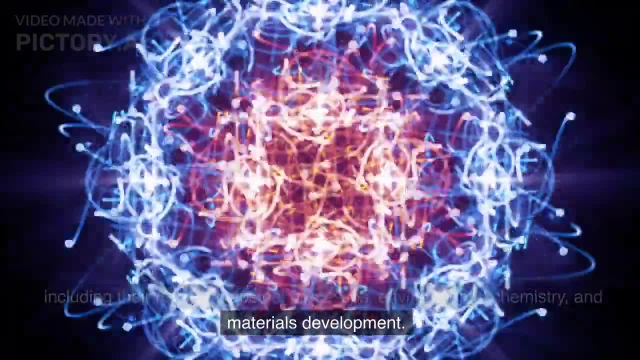 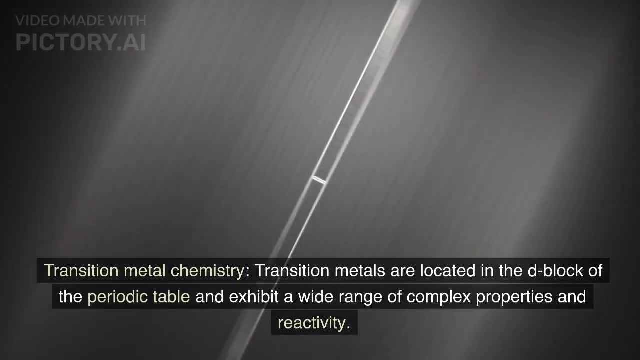 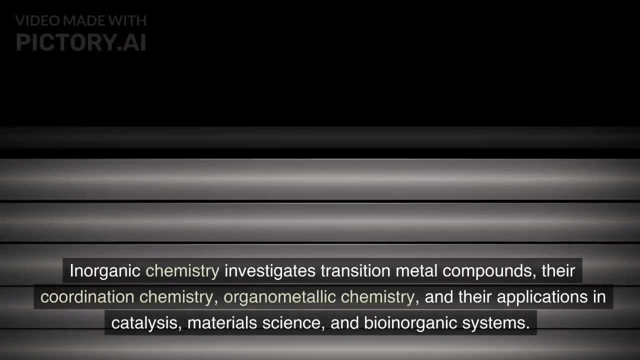 in industrial processes, environmental chemistry and materials development. 5. Transition Metal Chemistry. Transition metals are located in the D-block of the periodic table and exhibit a wide range of complex properties and reactivity. Inorganic chemistry investigates transition metal compounds, their coordination chemistry, organometallic chemistry and their 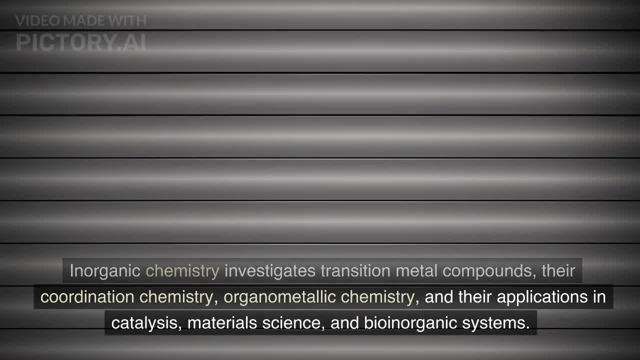 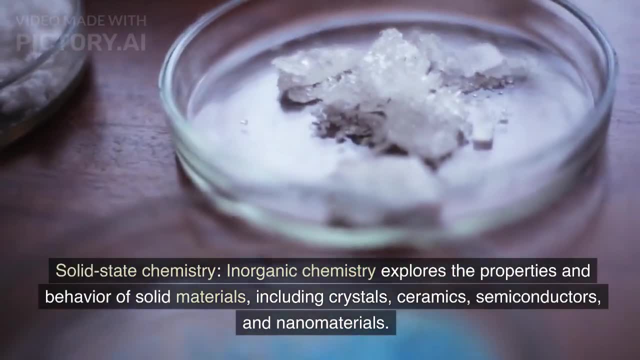 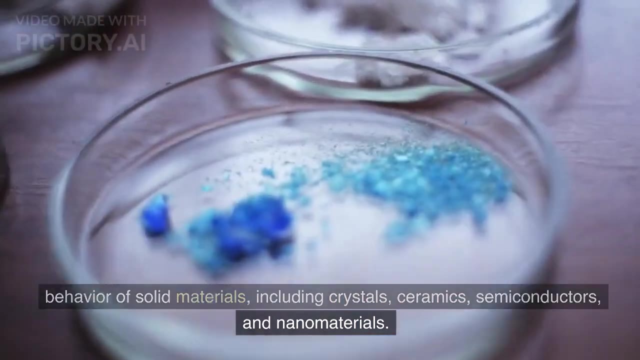 and their applications in catalysis, material science and bio-inorganic systems. 6. Solid State Chemistry: Inorganic chemistry explores the properties and behavior of solid materials, including crystals, ceramics, semiconductors and nanomaterials. It covers topics such as crystal structures, defects, phase transitions. 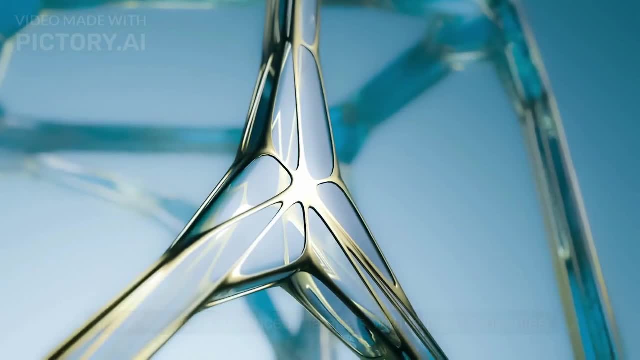 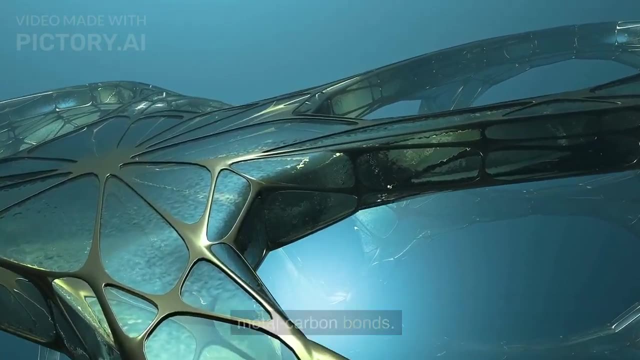 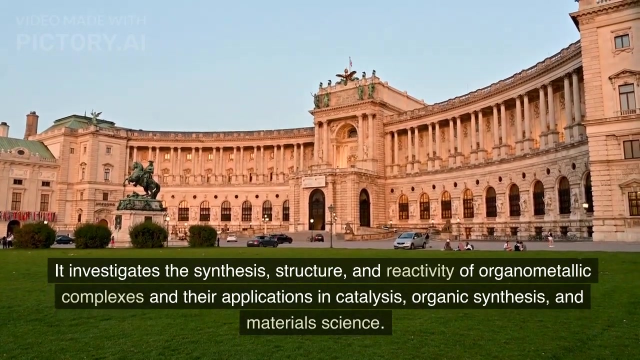 and the synthesis of advanced materials with tailored properties. 7. Organometallic Chemistry: This field examines compounds containing metal-carbon bonds. It investigates the synthesis, structure and reactivity of organometallic complexes and their applications in catalysis, organic synthesis and material science.